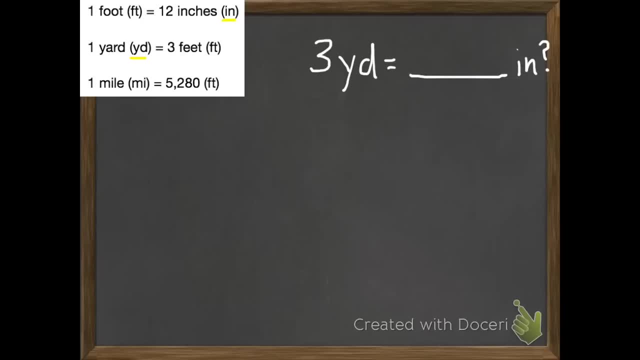 But we don't have a fact that goes from yards to inches, So we are going to have to use two of our facts to figure out a new fact. So let's start with our yards- One yard- and I break that into 3 feet, and then I can take each of those feet and turn them into inches. 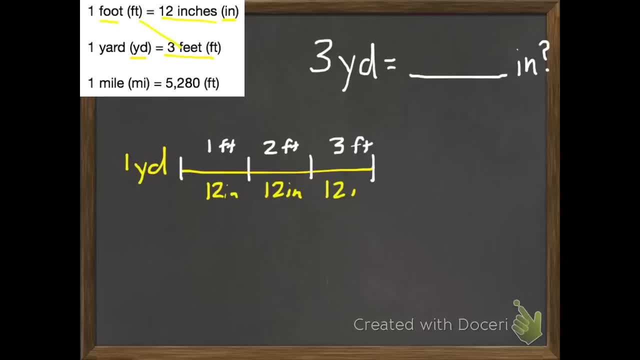 So each foot has 12 inches. So if we add up all of our inches, we have 12 plus 12 plus 12, or 12 times 3. That's going to equal 36 inches. So now we've created a new fact. 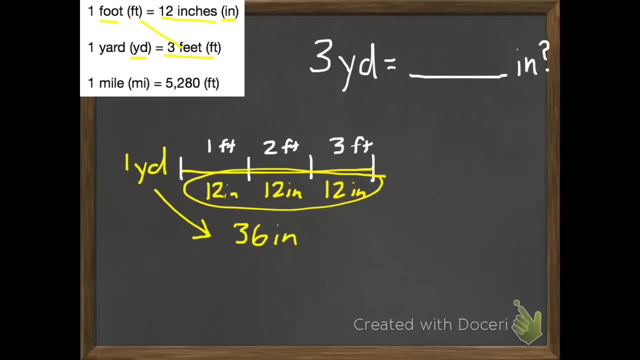 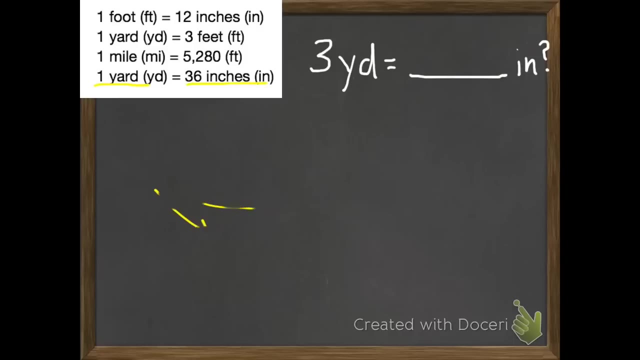 One yard. One yard equals 36 inches, So I'm going to add this fact to our little box in the top corner. So there it is, at the bottom: One yard equals 36 inches. Now that we know this, we can figure out our problem. 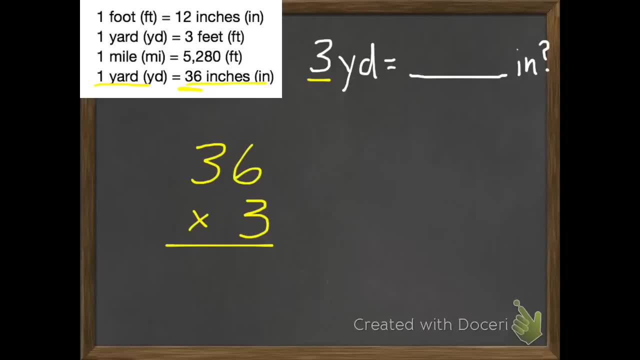 So we have 3 yards and there are 36 inches in each yard. So 36 times 3.. So 6 times 3 is 18.. 3 times 3 is 9, plus 1 is 10.. 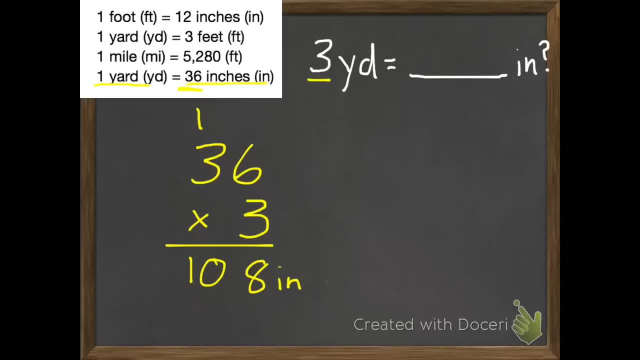 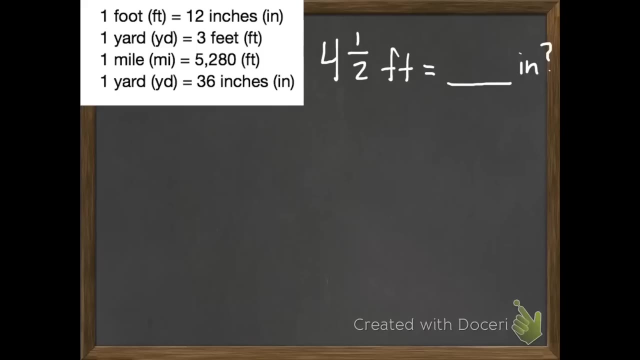 So we get 108 inches. So 3 yards equals 108 inches. I'm going to do another example So we can get an example of one of each of these. This one is a little trickier because I have a mixed number. 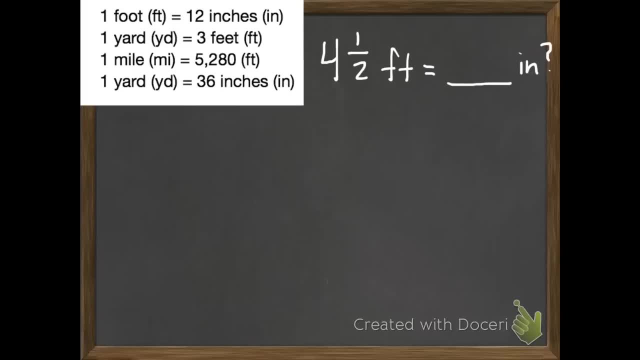 I have 4 and a half feet and I want to turn those into inches, So I'm going to break apart our mixed number. So I'm going to use just the 4 feet for now And we're going to use our fact over here at the top. 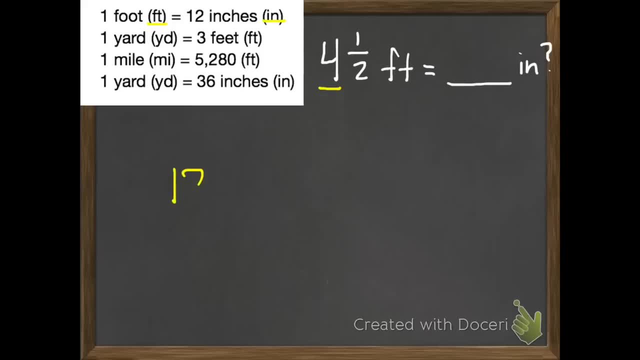 1 foot equals 12 inches. So if I have 4 feet times 12 inches, 12 times 4 is 48.. Plus just our 4 feet, we have 4 and a half feet. So I need to figure out this half of a foot. 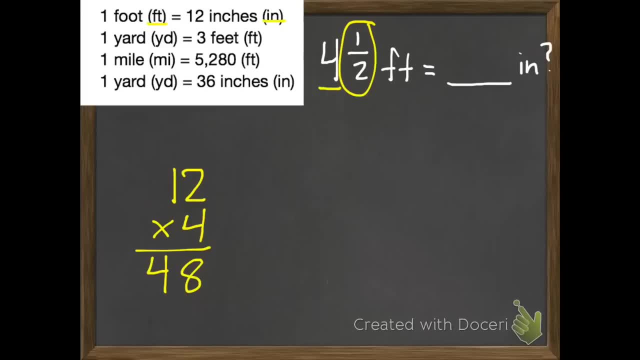 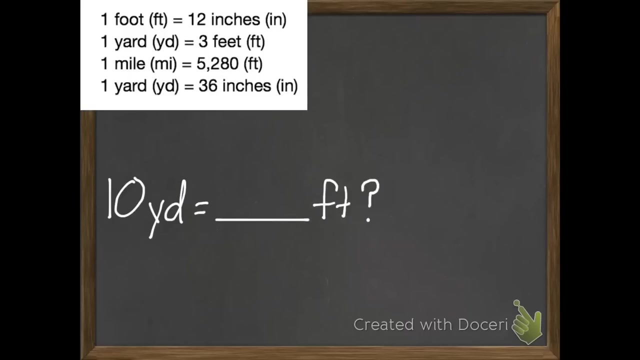 So if 1 foot is 12 inches and we have half of 12, that's going to equal 6 more inches, And 48 plus 6 equals 54. So 4 and a half feet equals 54 inches. One more example. 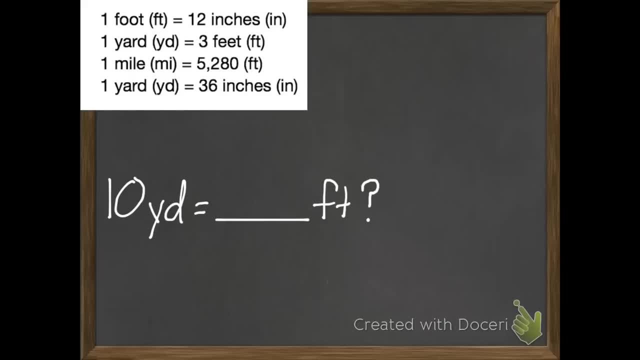 Actually, let's have you do this one. This one's pretty easy. So 10 yards equals how many feet? So first of all, we want to figure out which of our basic facts will help us in solving this. So do we have one that has both yards and feet in it? 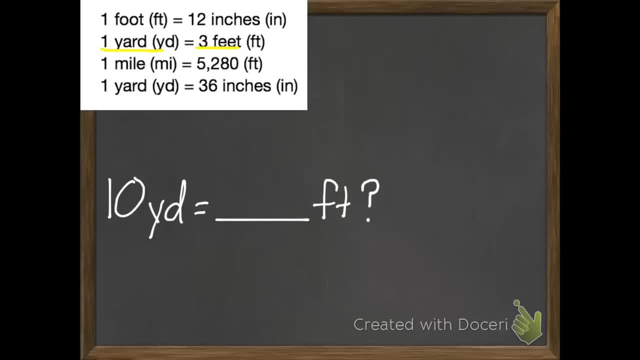 We do So, 1 yard equals 3 feet, So every one of those yards is going to have 3 feet. So what multiplication problem can you use to help convert 10 times 3, which equals 30.. I want you to try two more with me. 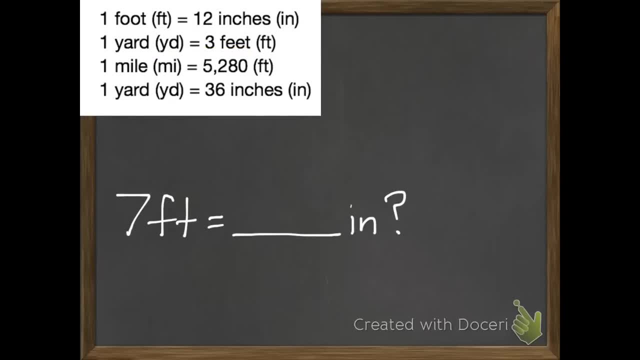 7 feet equals how many inches? First of all, again, we want to see which of these basic facts will help us. So this one has feet and inches. So 1 foot equals 12 inches And we have 7 feet. 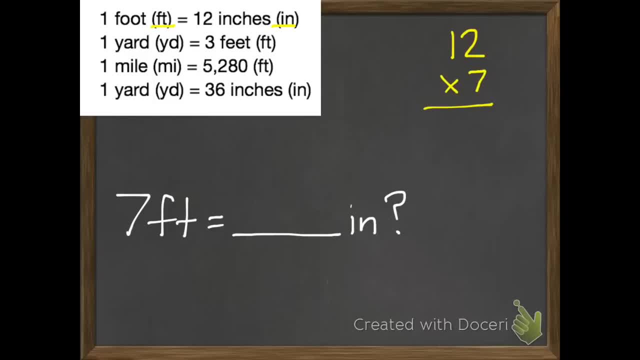 So that's going to be 12 times 7.. I'll give you a second to figure out what 12 times 7 is, and then you can check to see if you got it right. Okay, it's 84.. One last one to do with me. 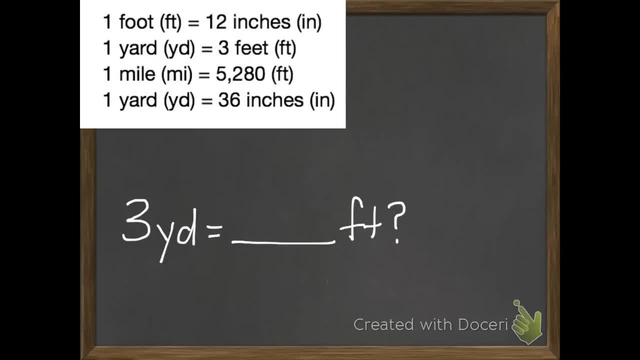 three or four problems. 3 yards equals how many feet? So we're going to use this one, which will just be 3 times 3, because 3 feet equals a yard and we have 3 yards, so 3 times 3,. 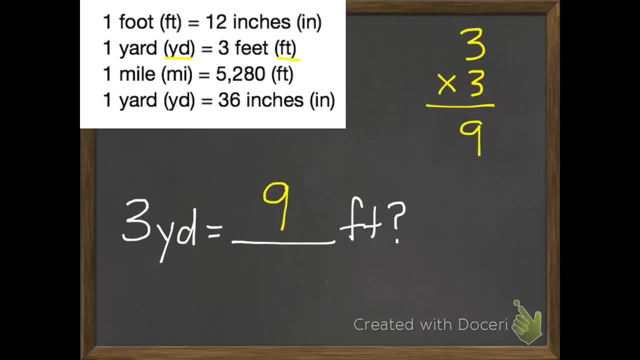 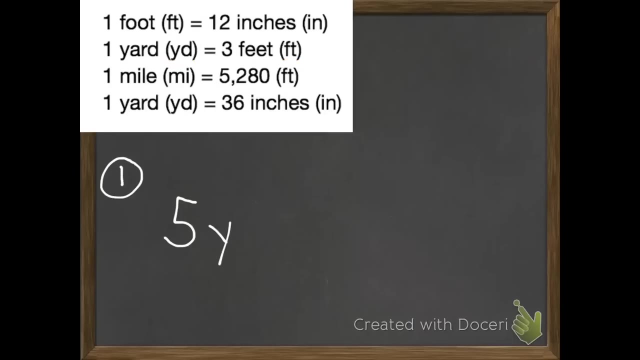 and that equals 9.. So 3 yards equals 9 feet. Okay, I think you're ready for your four problems. If you need to go back and watch any of these examples again, go ahead. If not, continue. So problem number 1..